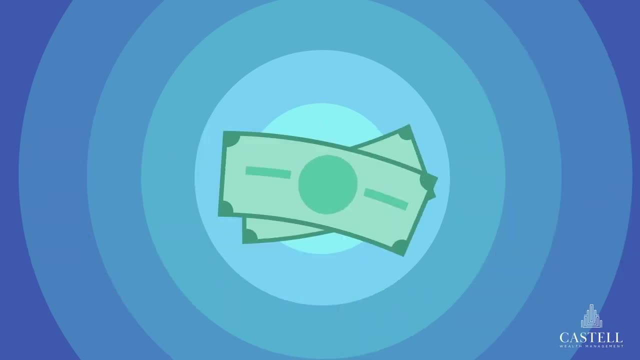 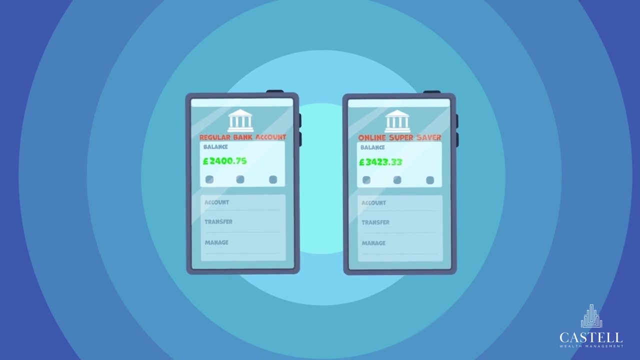 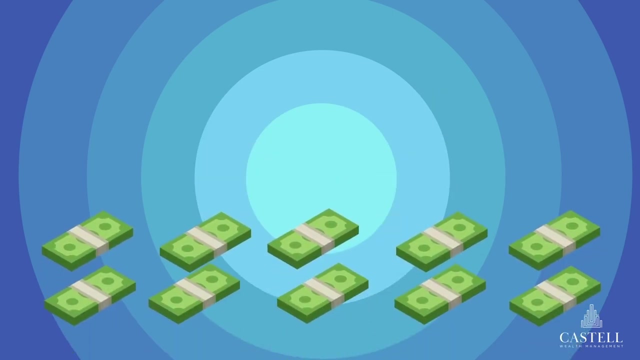 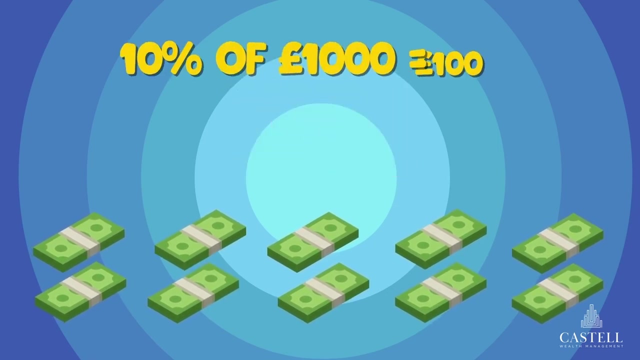 Compound interest helps your money increase over time and your money will grow at a faster pace than just plain old simple interest. Let me give you an example. He said: If you have £1,000 and you find a very generous, generous bank, that will give you 10% compound interest in the first year. 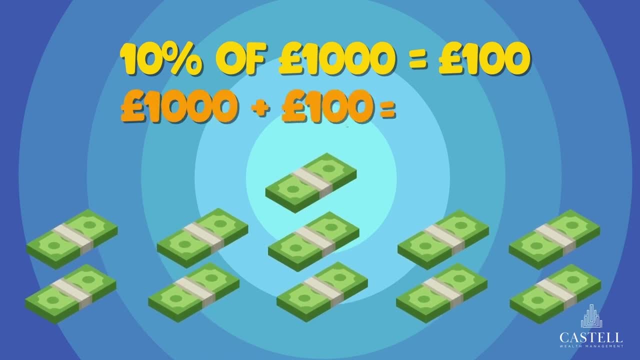 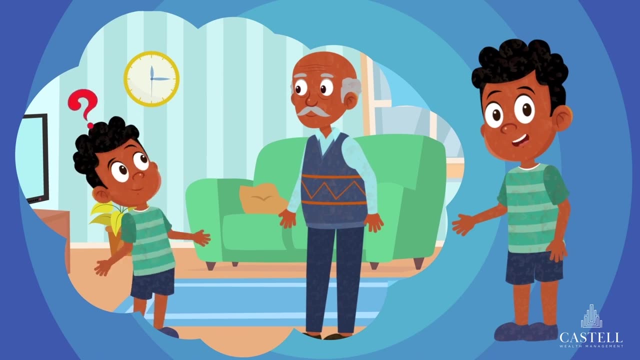 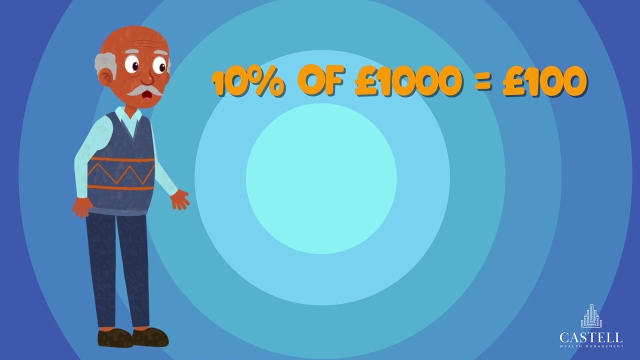 your money will be worth 1,100 pounds. My grandad saw my puzzled expression and explained a bit more Well: 10% of £1,000 is £100. So add it together and that means you have £1,100 in the bank. 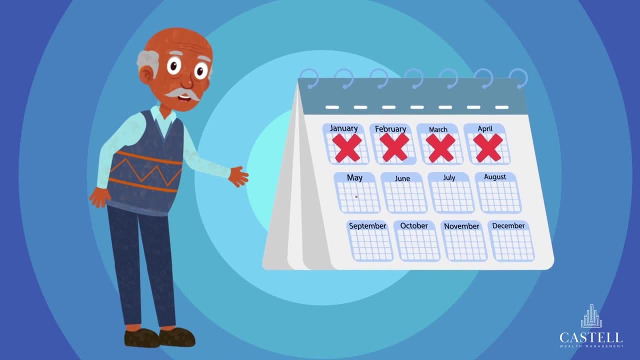 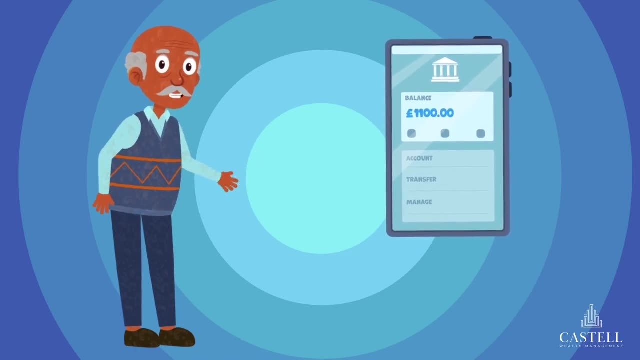 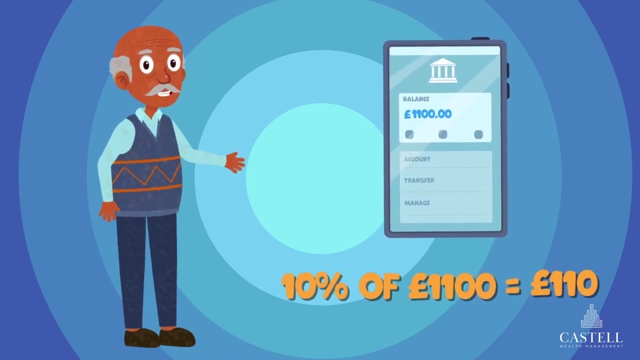 But here is the interesting part: The next year you have £1,100 in the bank, and so you get 10% interest on the original £1,000 and the £100 interest you made last year. So this year you get 10% of £1,100. 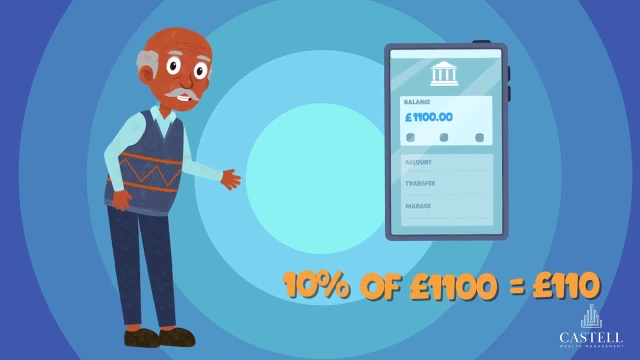 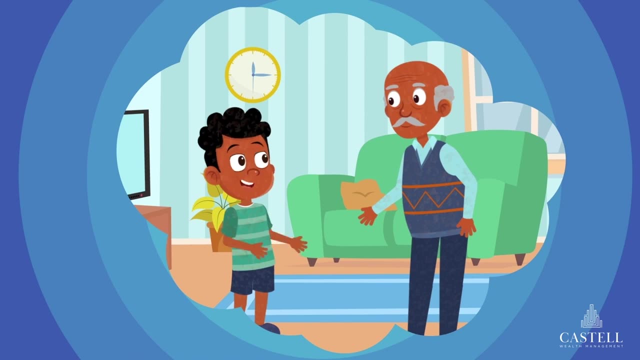 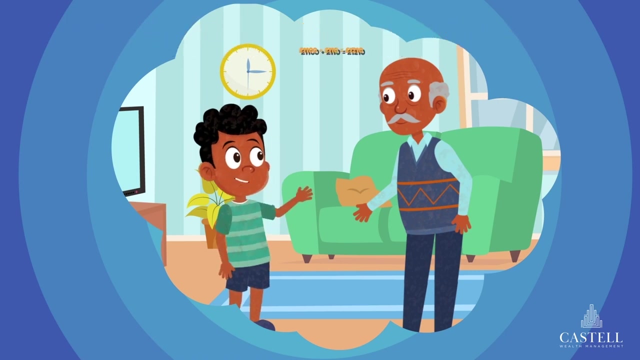 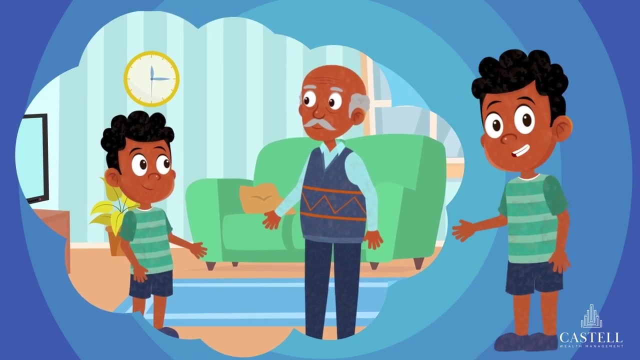 £1,100.. Basically the original amount and any interest you earned. Oh, now I get it. I laughed. Interest on interest. So does that mean you actually now have £1,210?? That's it exactly. my grandad chuckled. 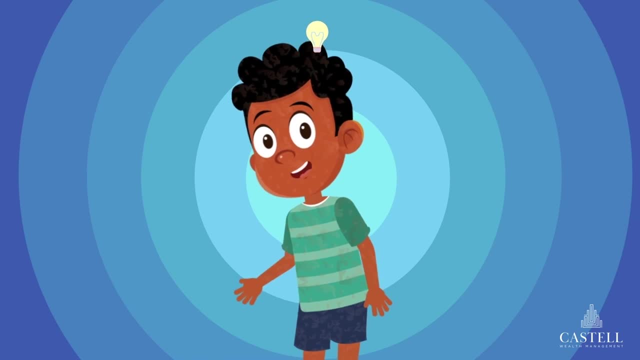 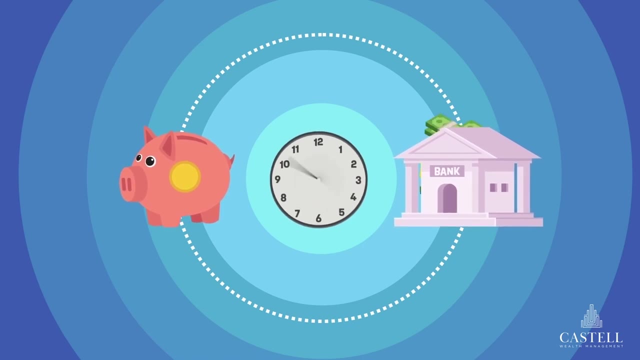 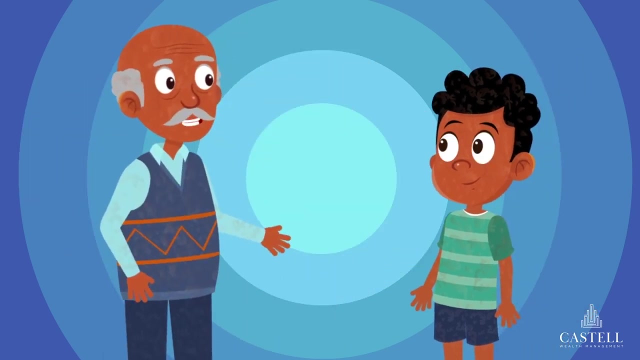 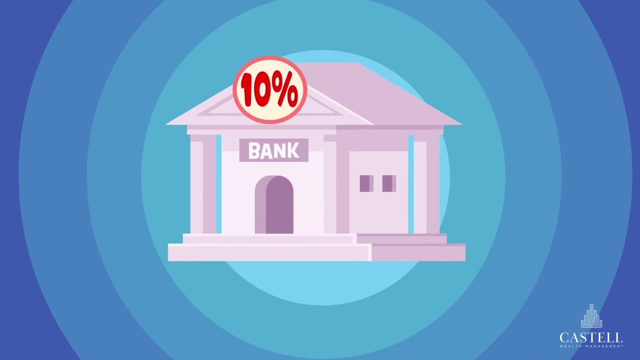 Hmm, I had an idea. So if I saved some pocket money and didn't take any out of the bank for a long time, it would be worth a lot more than what I put in. I asked. Correct grandad said It is important that you take note of the different interest rates that banks are giving you so you can find a good rate. 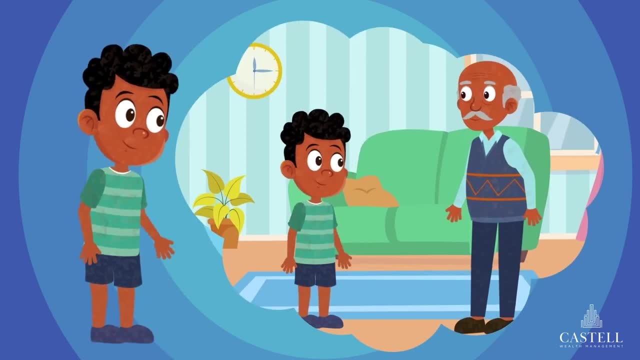 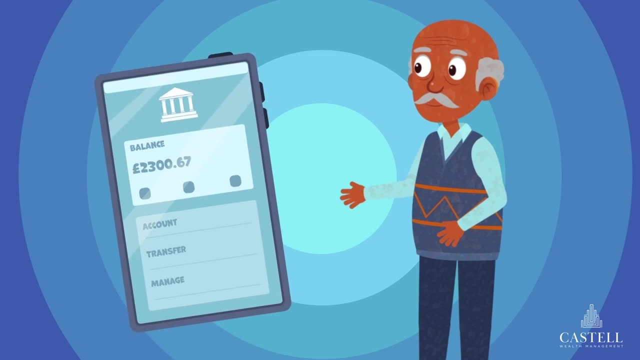 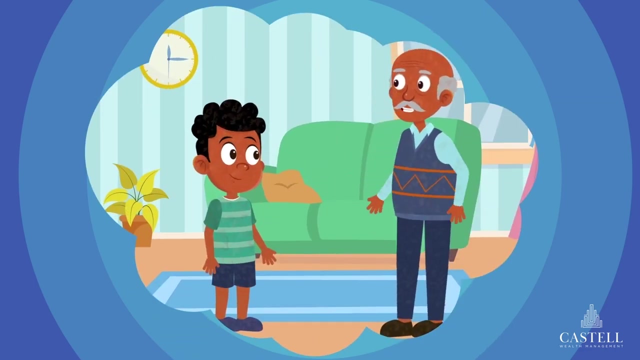 What does a good rate mean? I asked Great question, Jamal. my grandad said There are different types of savings accounts. like a bank account. This usually only gives a small amount of interest but is very low risk. Hmm, so that won't make as much money, I said.